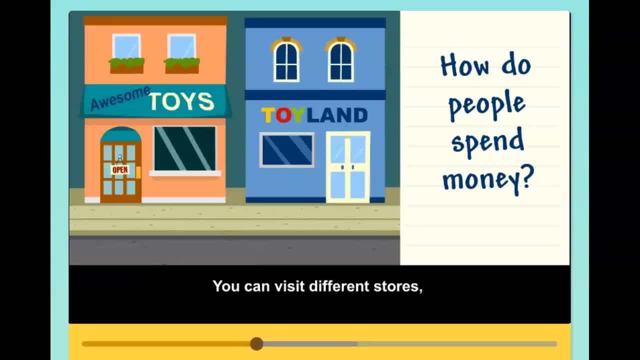 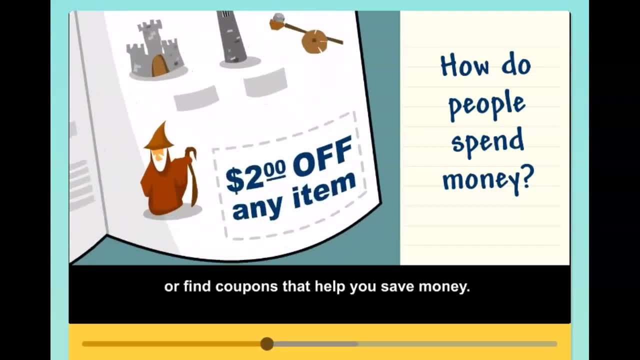 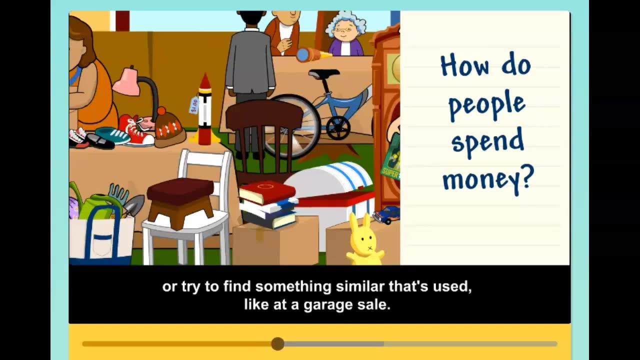 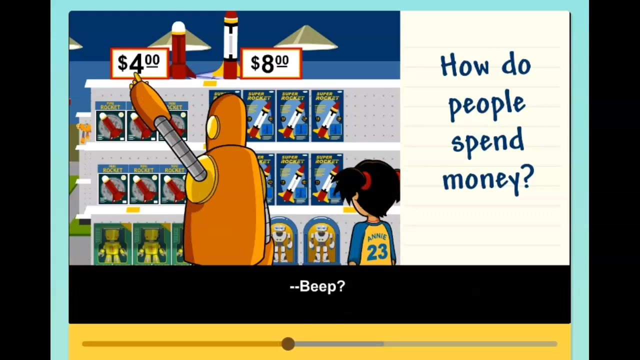 You can visit different stores, look online to compare prices or find coupons that help you save money. You can also wait and see if the price goes down later, Or try to find something similar that's used Like at a garage sale. You're right, Moby, this rocket's different, But it's cheaper. 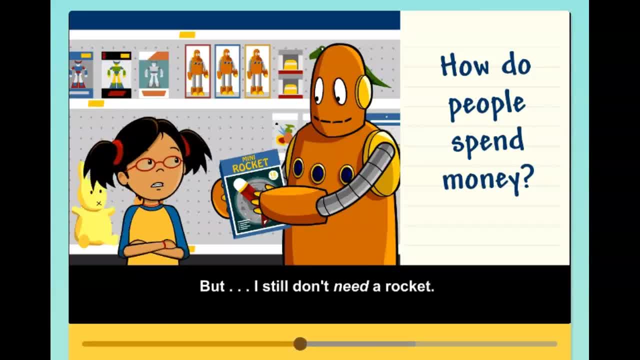 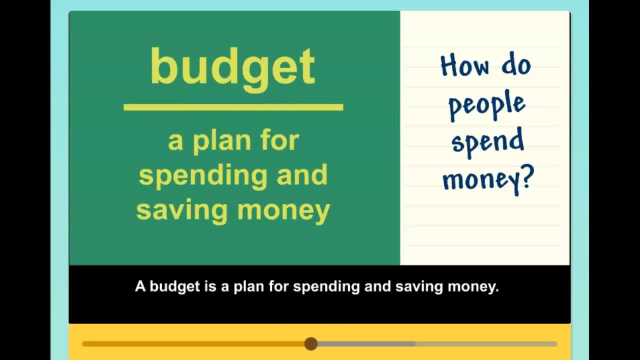 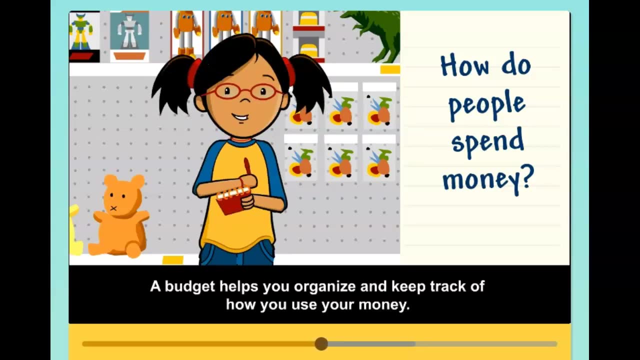 but I still don't need a rocket. There are other things I do need to spend my money on. A budget is a plan for spending and saving money. A budget helps you organize and keep track of how you use your money. My budget shows how much money I earned this week. 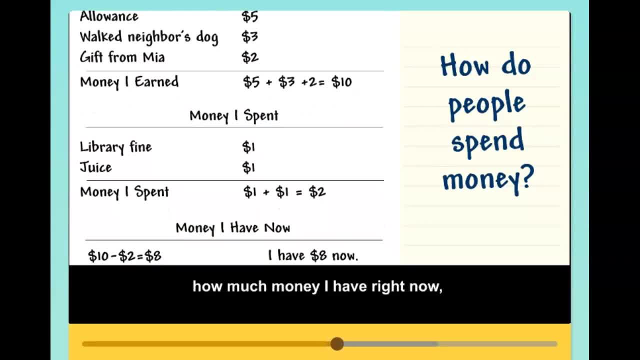 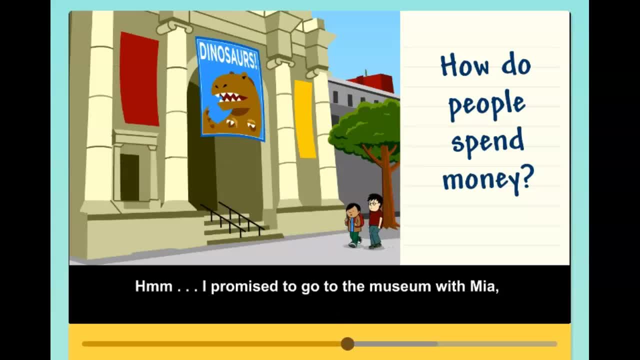 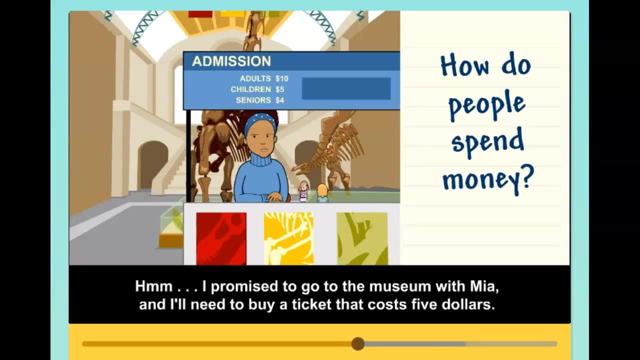 how much I've spent so far, how much money I have right now and what I need to spend money on. Hmm, I promised to go to the museum with Mia and I'll need to buy a ticket that costs $5.. If I buy that rocket, I won't have enough money left for a ticket. 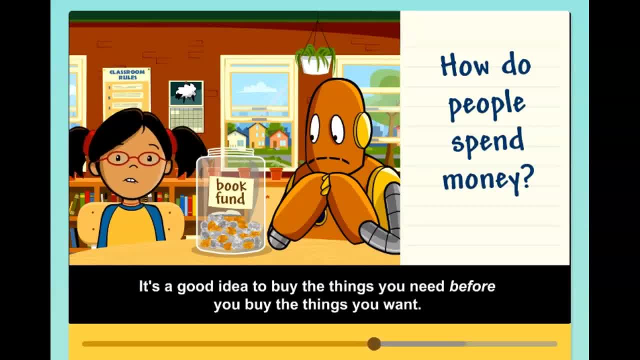 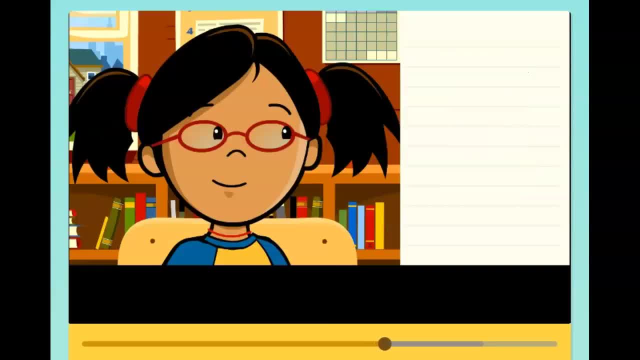 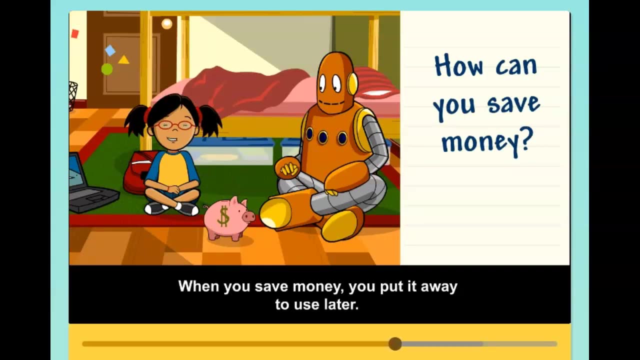 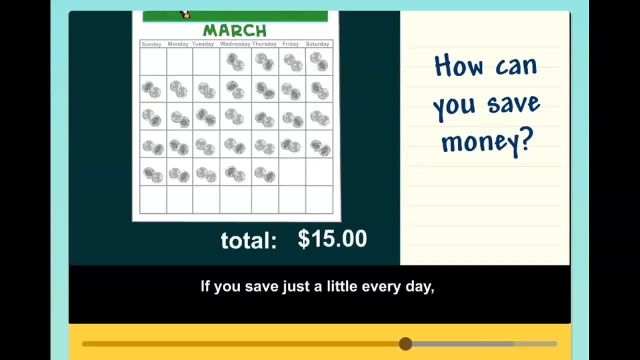 It's a good idea to buy the things you need before you buy the things you want. I'll save up money and buy a rocket later. How can you save money When you save money you put it away to use later? If you save just a little every day, you can save a lot in a month. 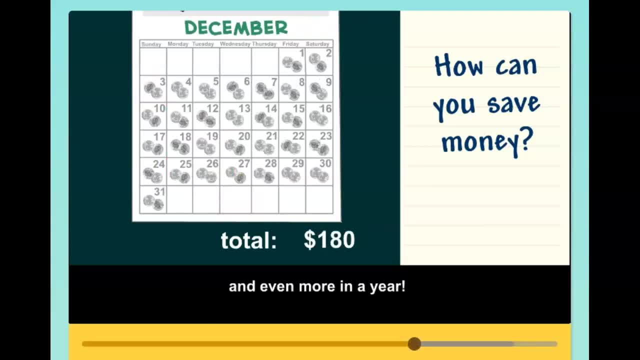 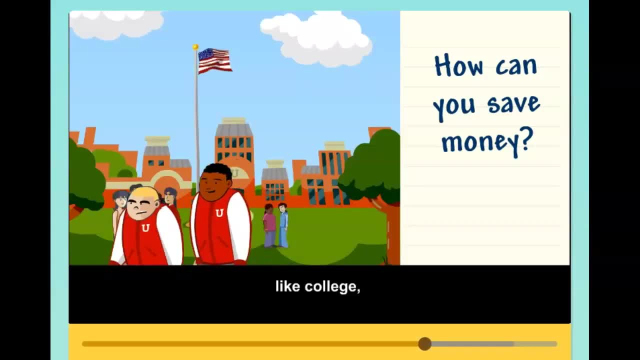 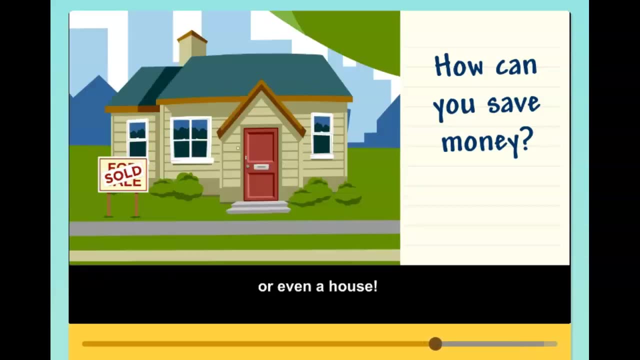 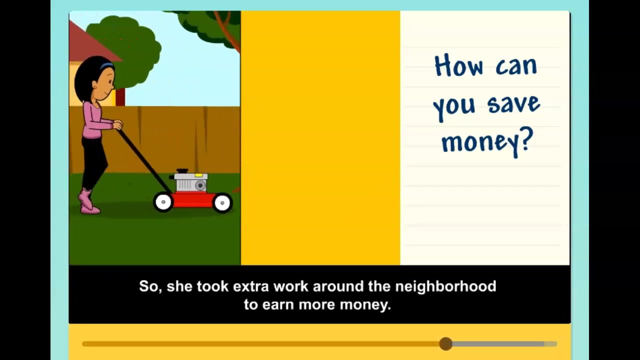 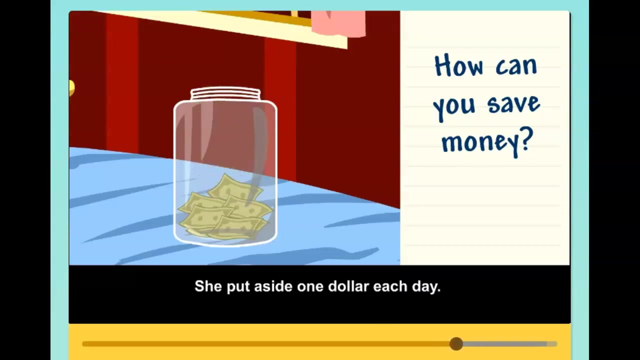 and even more in a year. A budget can help you plan for important things in the future like college, A car Or even a house. Mia really wanted a guitar, So she took extra work around the neighborhood to earn more money. She put aside one dollar each day. 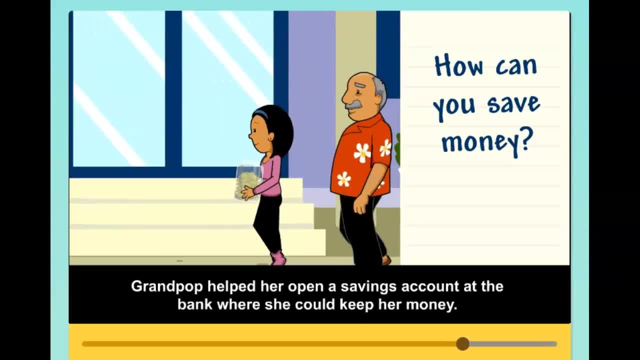 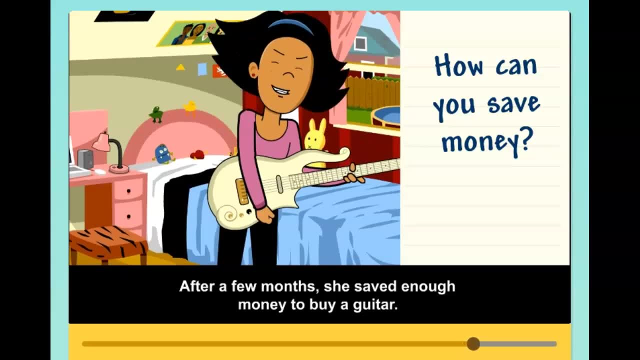 Grandpop helped her open a savings account at the bank where she could keep her money. After a few months she saved enough money to buy a guitar And now she can play the guitar. Maybe we should save up to buy some earplugs.